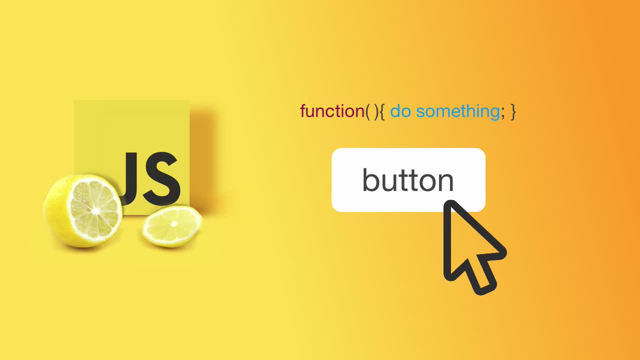 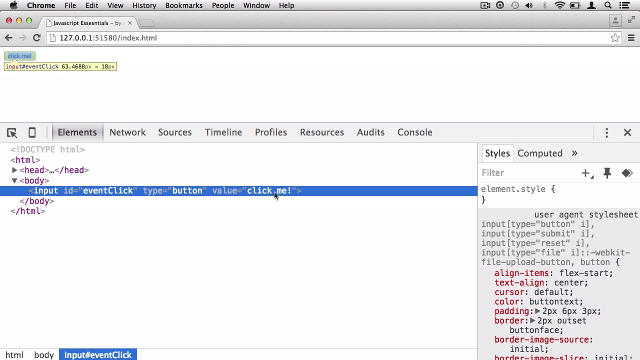 specify. We create that function and we say: if they click a button, I want to go ahead and perform an action, And that's how we create interactivity. So we're going to start out with a very simple example. So we have a basic input right here. It's just a button with the value of click me. So we just have this. 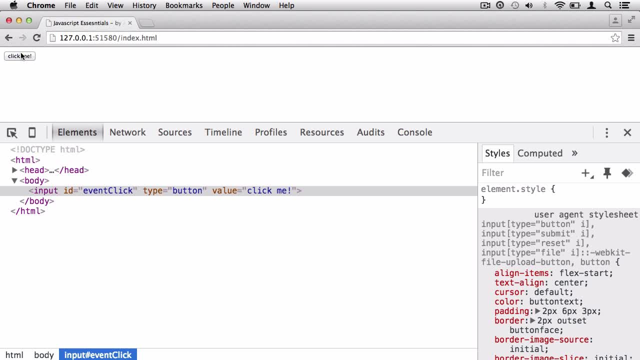 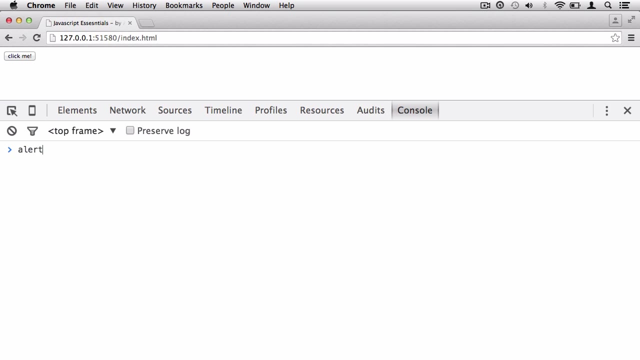 nice little button right here and it doesn't have any functionality. But when I click on this button, what I want it to do is bring up an alert dialog box. So first of all, we haven't discovered how to create an alert dialog box in JavaScript, which is very easy to do: Just type in alert and then you. 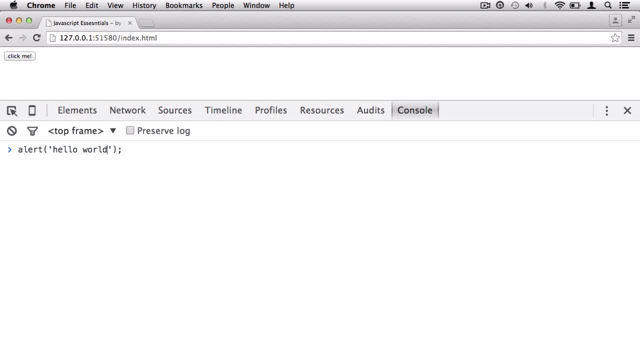 can click Oncetag virtually and this will show up inside of the dialog. So this is how easy it is to create an alert dialog box in JavaScript. So notice, when I hit return and execute this command, an alert dialog box will show up and it has the string hello world inside of. 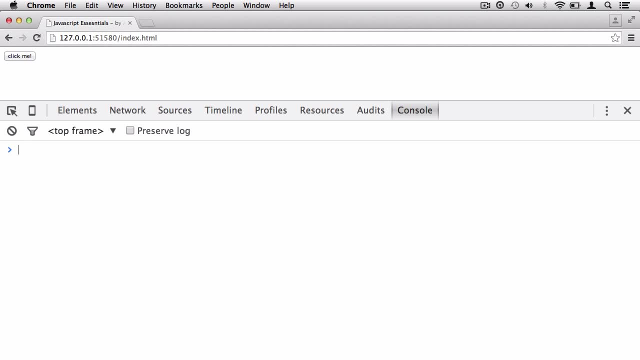 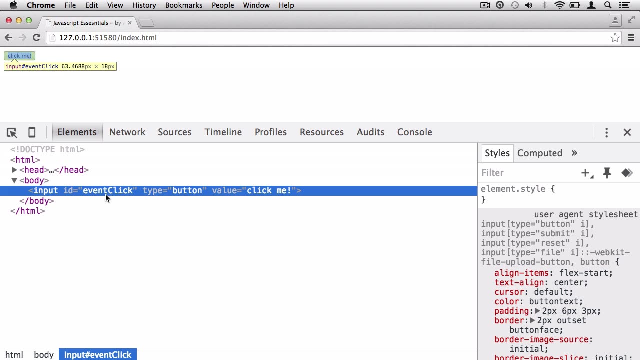 there. So that's nice and easy. That's how we create an alert dialog. Now I want to first of all target this DOM element right here is via its ID. So this DOM element has an ID with the value of event click, So we know that we can. 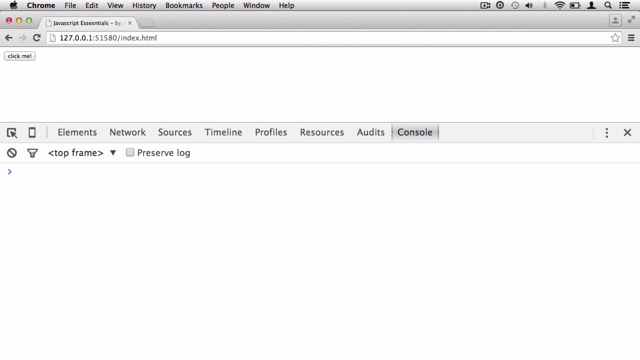 target this specific element via its ID. So I can say documentgetElementById and we want to get the element which is going to be event click. Now I want the console to print out a JavaScript object. So I'm going to wrap that inside of the DIR function. And if we take a look at this now, 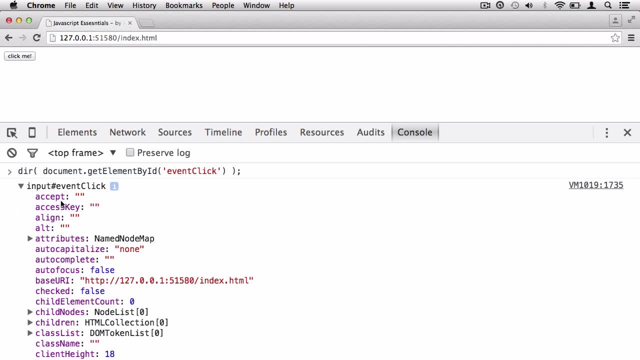 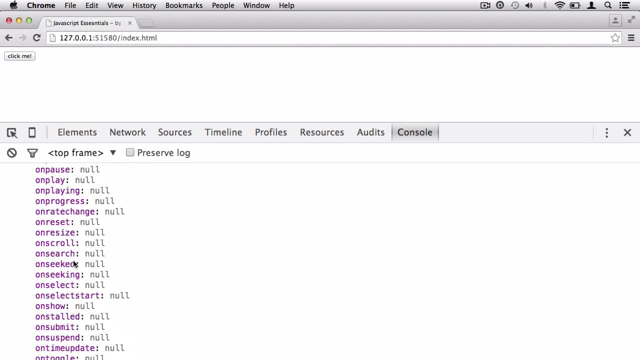 here is the JavaScript object that represents this DOM element And we can take a look at all of the events right here. And again, we can tell that these are events because they have the on word in front, So you have on focus on error and so forth. Now most 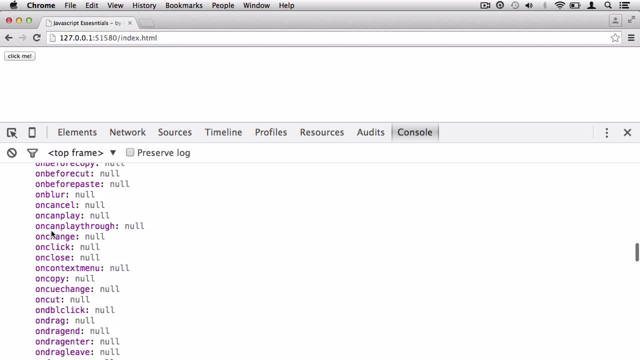 of these events may not even actually really apply to this element, but JavaScript does allow you to attach all of these events, but some of them won't apply. For example, you have, let's say, if we go down. you have, let's say, on play, on pause, and so forth. These right here are more for the HTML5. 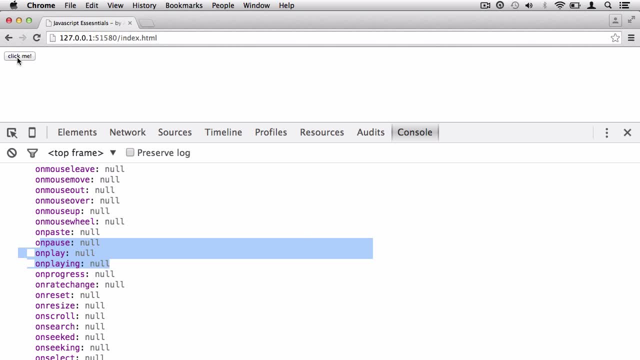 video element, but they are available on this button, but it's not really ideal. Those are just for the HTML5 video element. So I'm going to take a look at this and I'm going to see why those events won't be triggered on this type of element. So what you have to do is you have to look at the element. 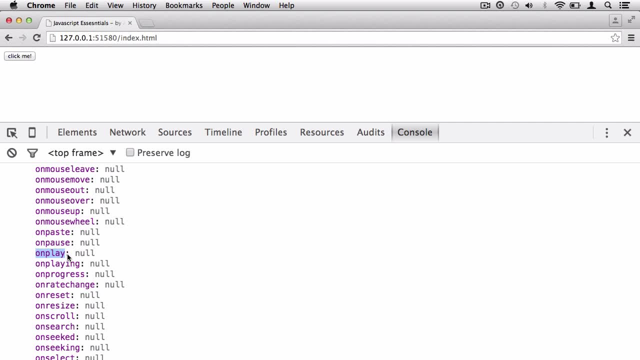 and say: does it have that functionality? Can you play a button? No, you can't. Can you pause a button? No, you can't. So those events, you are better off just leaving null for this element. But for example: 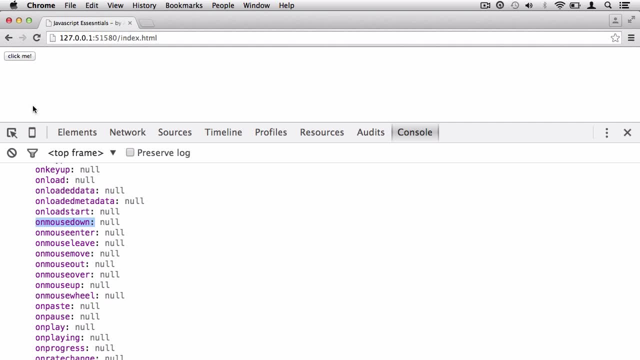 can you, let's say, on mouse down. So when I push my mouse down, is there an event triggered there? Yes, On mouse out, for example, And even on mouse over, if I can make a mouse go up, then I'm going to be able to see which elements are triggered. And again, 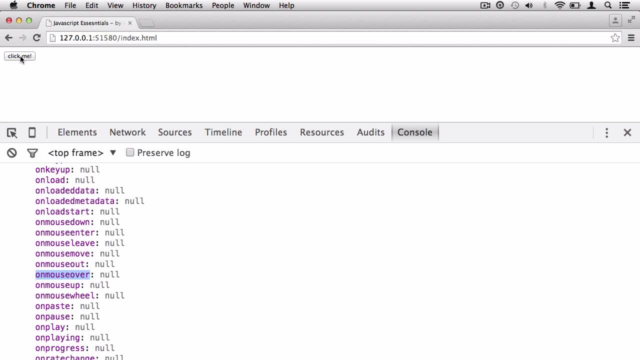 If I hover my mouse over this button. yes, that could trigger an event. OnMouseOut is when I'm holding down, so the event won't trigger. And as soon as I release, then the OnMouseOut event will execute. So you have all of these events. 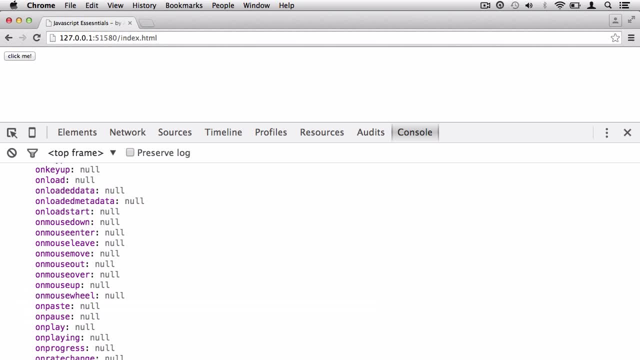 You just need to look at those events and you need to decipher can those events be triggered on this type of element. But we're gonna keep things real simple and we're just gonna go with the standard click event. So when the user clicks on this button, 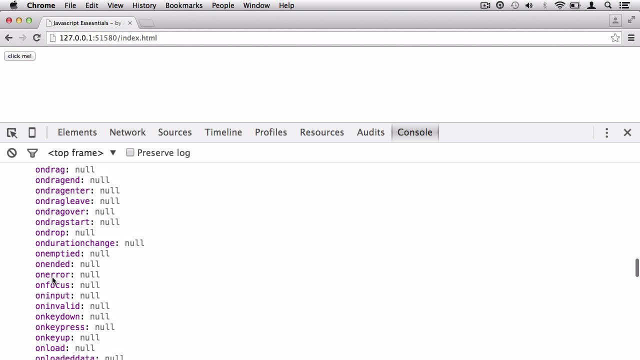 I want to trigger an event, So let's go ahead and take a look at the onClick event, which should be in here. There it is onClick. Now we know that this event isn't going to trigger on this particular element because its value is null, right here. 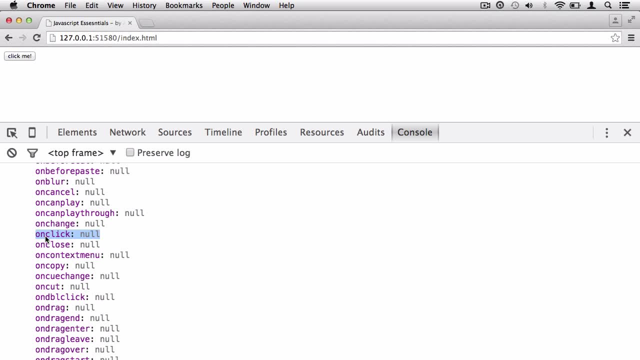 So at the moment, onClick is not defined, So let's go ahead and define this event. So the first way of attaching an event listener is to attach it directly via this object right here. So I want to again target the document. 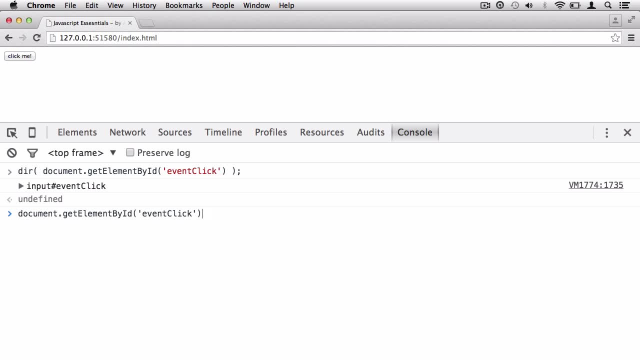 which is JavaScript's representation of a HTML file. We want to pull out a specific object to do with an element with the ID of event, click, which will return this object, as we know, And then what I want to do is- as we're working with an object now, so don't forget- 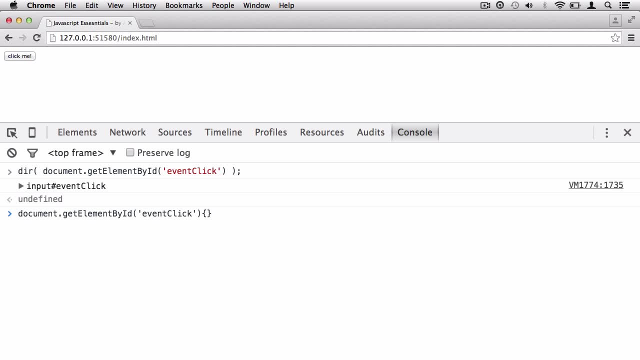 this is just pulling in this object. so we are working with an object. I can just say onClick. Now I am targeting the onClick property right here on this object and I want to change this from a property because at the moment it's null. 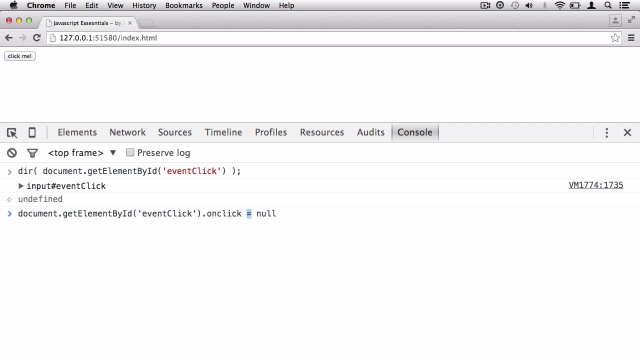 which means it contains a primitive. so it's a property and I want to reassign the value to be a function. so now it's a method And this is going to be triggered. this function right here will be triggered when we click on the button. 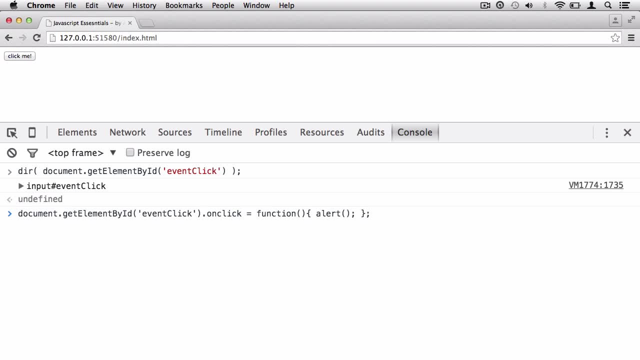 So I'm just going to create an alert dialogue, So I'm just gonna say alert and then I'm gonna say hello world, Very simple. So all I'm doing is I'm targeting that object, I'm targeting on click and I'm reassigning the value. 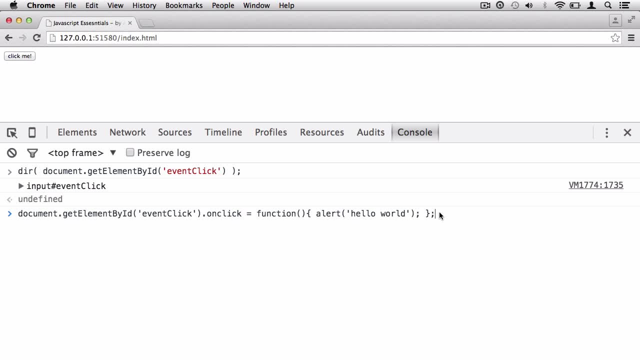 So I'm deleting that null value and assigning a function in its place, And this function is simply going to open up an alert dialogue. So now let's go ahead and pull up this object again. So I'm just gonna do it in the DIR function, don't forget. 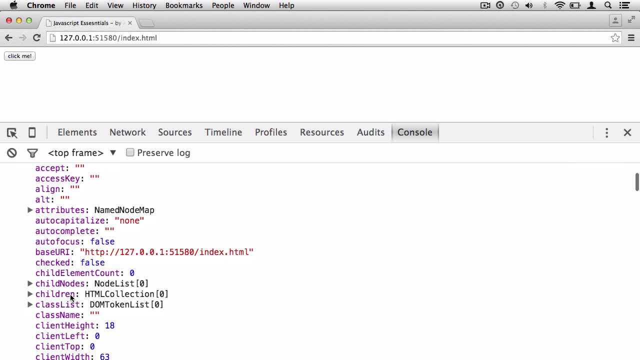 So I get an interactive list And if I scroll down and we go to on click, you will notice it is in fact a function right there. So let's see if this function executes when we click. So I'm gonna click on the button. 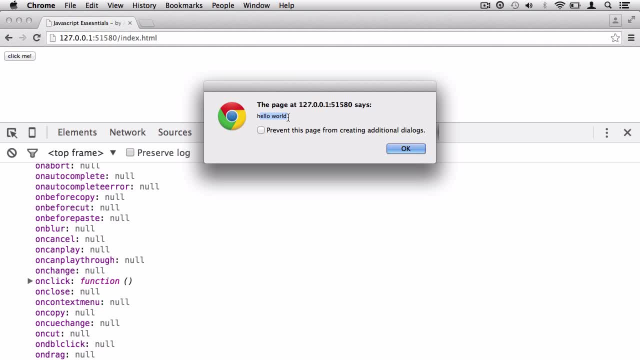 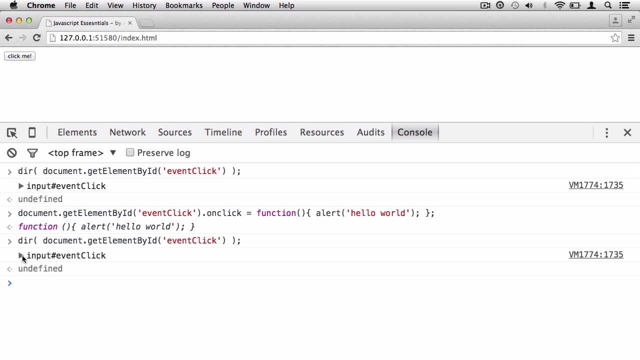 and there you go. You now have an alert dialogue box and it has the string hello world. That's exactly what I told the function to do. So this is one way of adding an event listener. Now there is another way that adds an event listener natively. 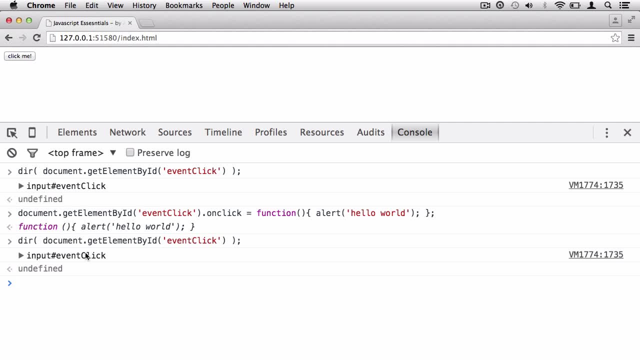 And this is ideally the way you should do it. Not this way, but by using the add event listener method. So what I want to do is refresh. Refresh the page, And now what I'd like to do is print out the object again. 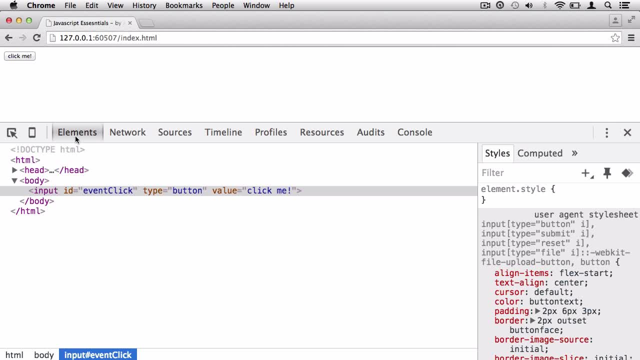 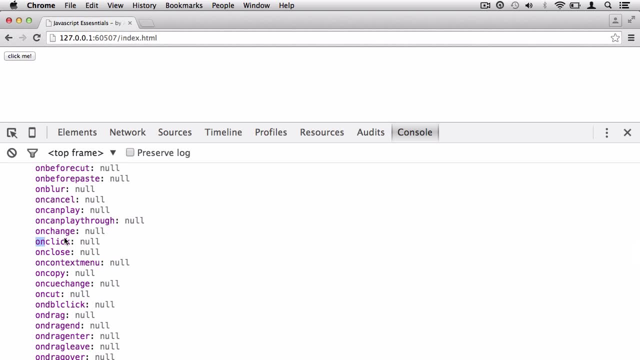 to do with this input element, that we have this button And you'll notice that dot on click or the on click property will have the value of null. Likewise, I can just say: you know, go grab that property and return the value. 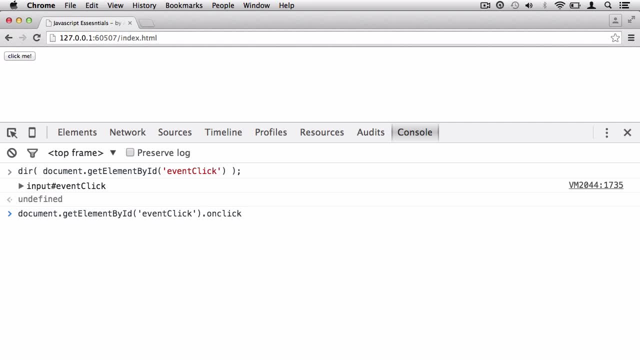 for example, dot on click And that will tell me if that particular key name stores any values, which at the moment is only storing a null value. So now, when I click, nothing will happen. All those events have been completely removed, or that particular event has been removed. 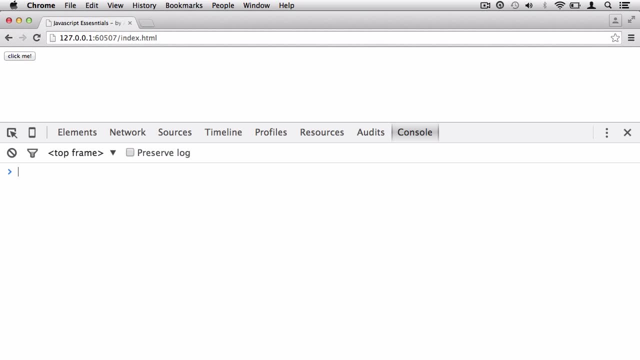 But what I want to do now is add an event listener natively. So again, we do exactly the same thing. Whenever you want to work with a specific element, you first need to target the object that resembles that element in the document And then you need to say: add event listener. 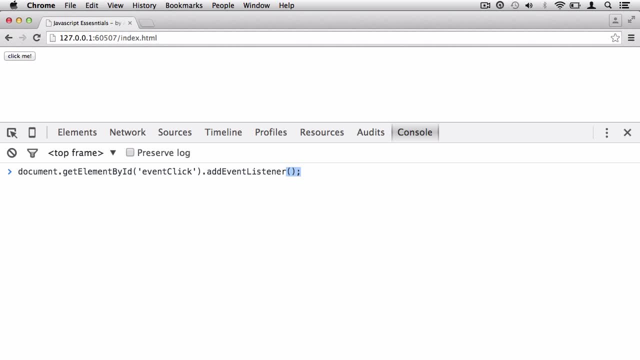 and then we need to pass in some parameters to this method. Now again, be very, very careful here. Events must have a capital, E and L must be capitalized as well. And then we need to first of all pass in a string. 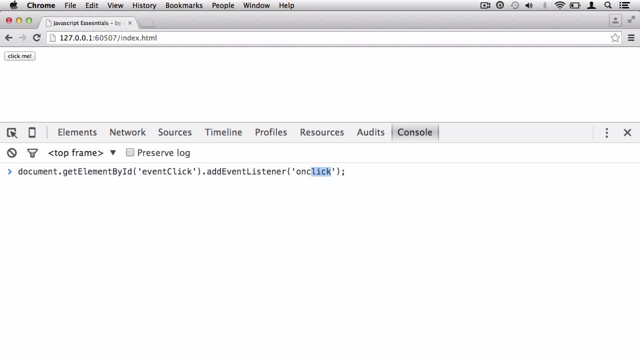 Now we don't say on click anymore. That is the property name on this object, That is a key name on this object. However, when you want to add an event listener, just omit the on, so get rid of on And then you're just left with the actual event name. 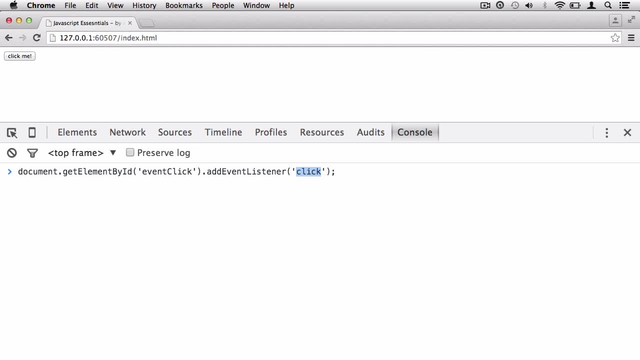 which is click, So you can have a look through all those different events that you can apply and just omit the on word in front of it. So that's the first parameter, which says that's the event that we want to add: a click event. 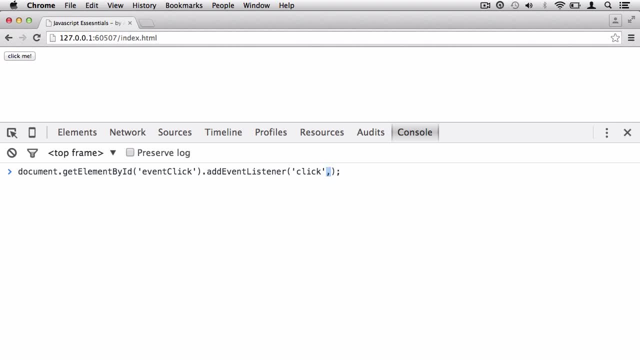 Next, we need to define a second parameter, So we need to put a comma in here, and then we need to define a comma, And then we need to define the function, which, again, this is going to be the function that is invoked. 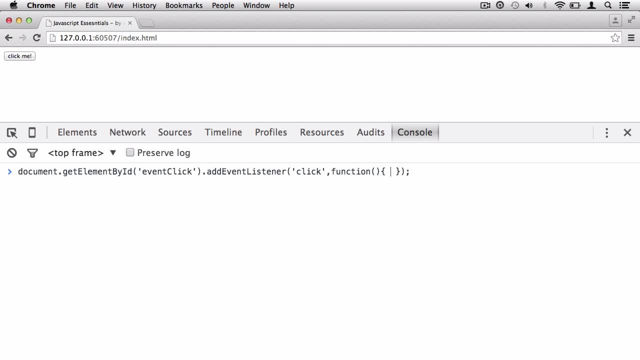 is executed when that event is triggered. So let's go ahead and create an alert dialogue box with the value of hello world, exactly as we had before, And if I go ahead and click, you will notice that it shows up. here There's the alert dialogue box that I told it to bring up. 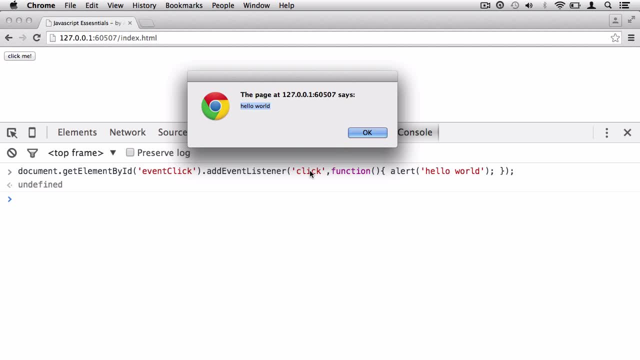 when this event was triggered, It has the string hello world inside of it. Now the difference is: let's go and take a look at our object that resembles this DOM element. So again, I'm just going to put that into the DIR function to get an interactive list. 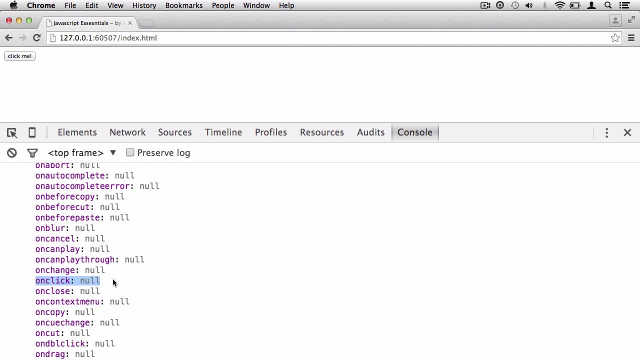 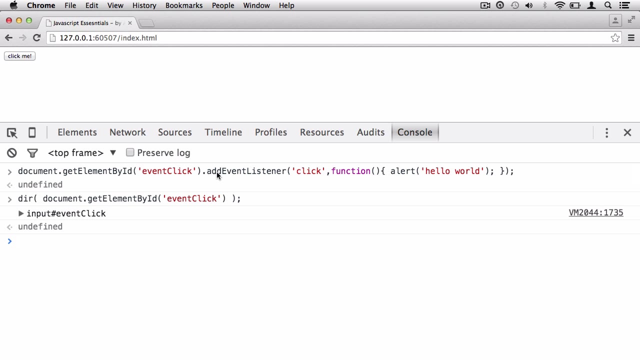 And we scroll down and on click is null. Now that's kind of strange, because last time it was a function and we knew that when we clicked it that function got invoked. So where exactly has this event listener right here added this function? Well, the simple answer is: you can't actually look. 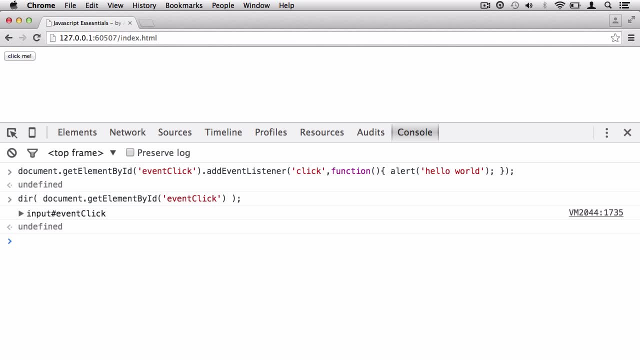 at this particular event because it's managed by the native code. Now, how do I know that? Well, the simple answer is: I'm going to target the add event listener, but this time I'm not actually going to invoke this function. So don't forget this. right here is a function. 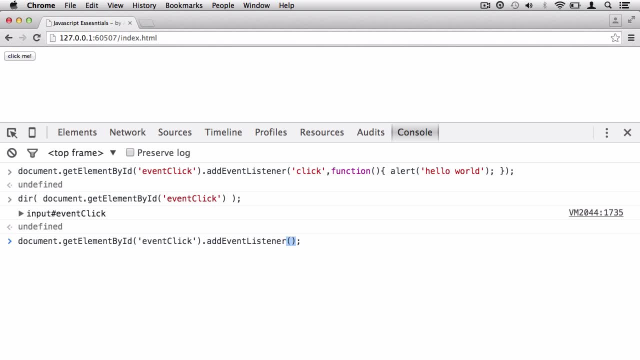 the add event listener function, but I don't want to invoke it Now in JavaScript. what you can do is say no, don't invoke it, don't run it Rather if you don't include those brackets, as you know. 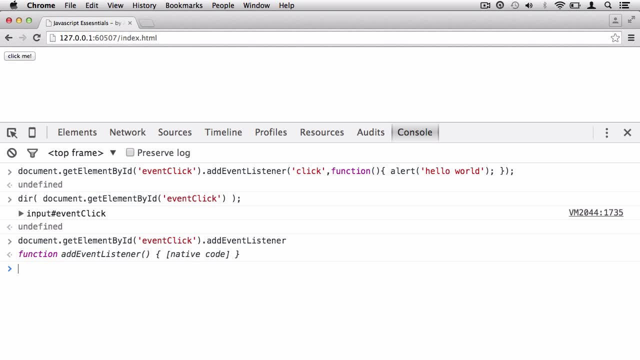 it will return the function text, So we can actually look at the function itself in syntax. Now you will notice something quite strange here. It gives you the function name: add event listener. Yes, that's fine, But wait a minute. what's this? 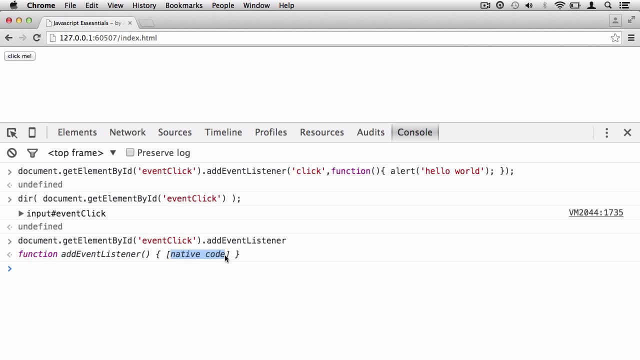 This is native code. This means that this function is actually running code in terms of the JIT compiler. It's actually in the programming language of the compiler, which is a lower level language, which is CPP, If you don't know what I'm talking about right here. 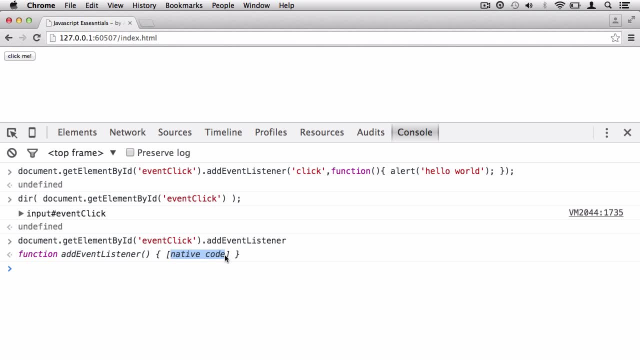 don't worry about it. It's native code that you can't look at in JavaScript, So those instructions are written in a different language, essentially. So what happened with our event listener? Well, this event was actually written in JavaScript. It's actually attached natively. 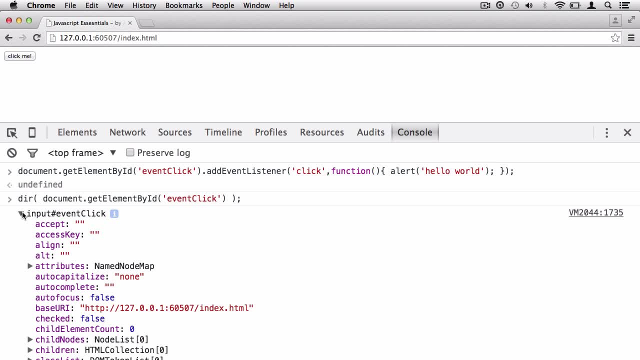 So that's different. Before I was attaching an event directly on the object itself and we saw that function. but now this is actually being handled by the native JIT compiler. So we can't actually look at our event now in an actual sense of, you know, printing out an object. 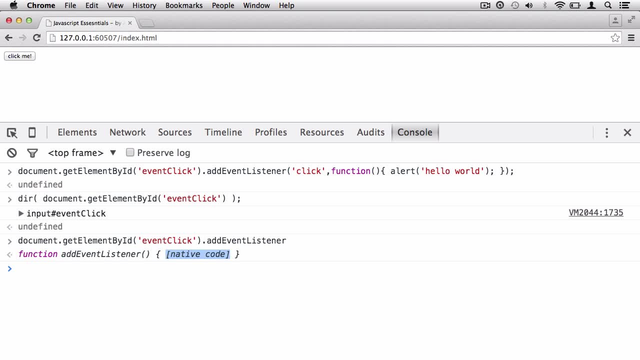 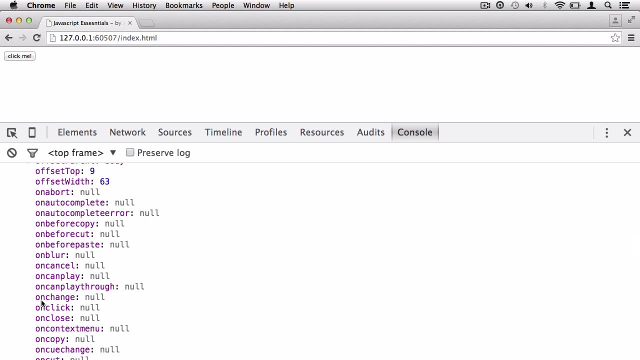 and looking at where that function was produced. This is all being managed natively And therefore that's why we don't have to do that, And therefore that's why we don't have to do that. We don't have the onClick property right here. 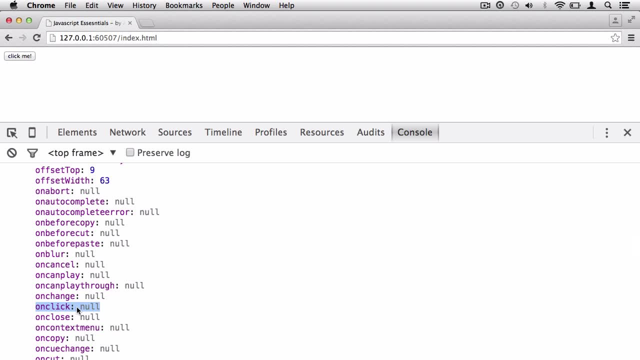 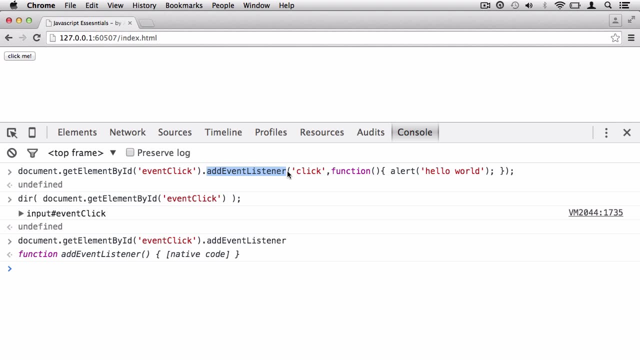 set to any value, It's still set to null. This is a different way of attaching an event listener, But, however, this is recommended because this is faster, So when we run. so when I executed this line of code, what it did was it told the JIT compiler. 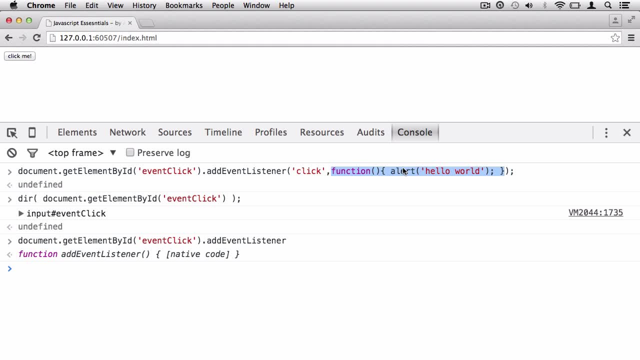 I want you to manage this function right here, Because what it did was it took this function and it converted it into native bytecode, And so that means the function has been interpreted and it's waiting for that click event to trigger, And so this is all happening in the native side. 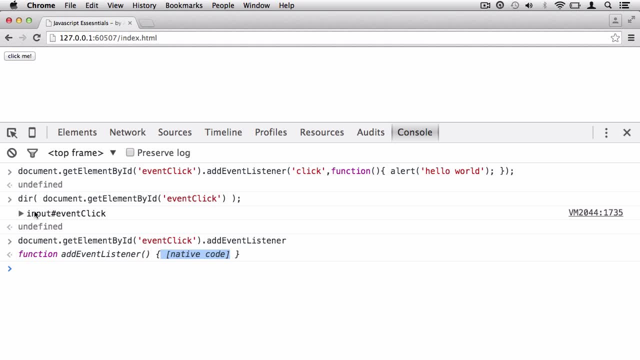 which is quicker, Whereas if we were to attach that function to the key name onClick, well, when the button is clicked it goes to this object. It takes a look at that onClick key name and it sees if it stores a function. If it does, then it takes that function. 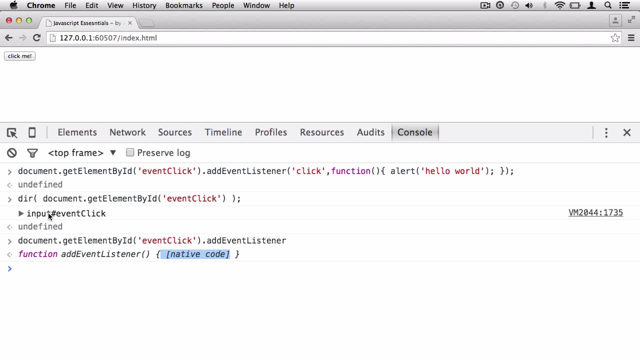 It then compiles the function and runs the function. It then compiles the function and runs the function. However, this way means that the function is already in native bytecode, so it's executing a lot quicker, And when you have hundreds of events on a page. 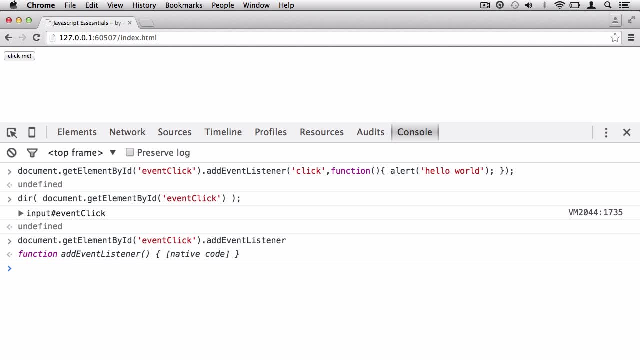 that could be triggering loads and loads and loads of times, thousands of times. then having your code already compiled, having that function ready and compiled and waiting to be executed, is a lot faster. Now also, there is another benefit to adding an event listener. 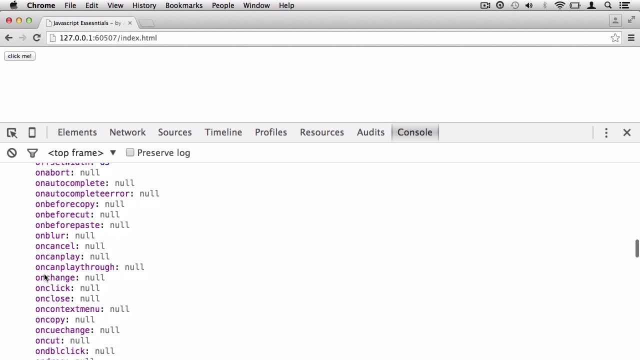 And that is, if you take a look at the onClick property, this key right here, and you, let's say, populate that key with a function, turning it into a method, then you could only have one function in that key, which means you can only have one function. 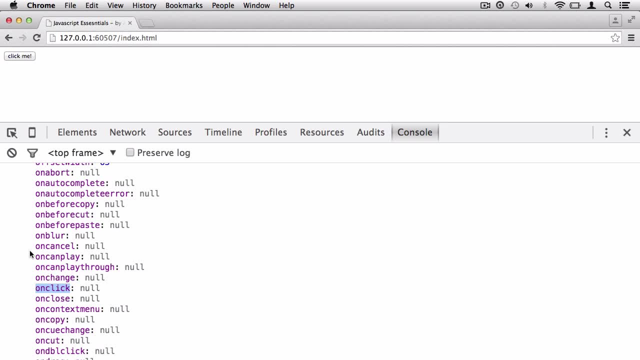 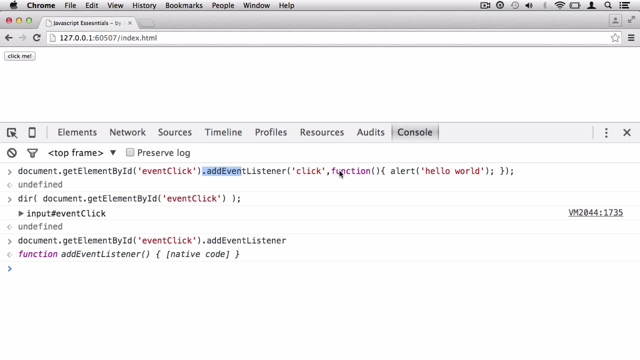 that executes when the button is clicked. However, in the case of the addEventListener, you can actually have multiple events. So here's the first one that we added, which was a function that brings up an alert dialogue. So here's the first one that we added, which was a function that brings up an alert dialogue. 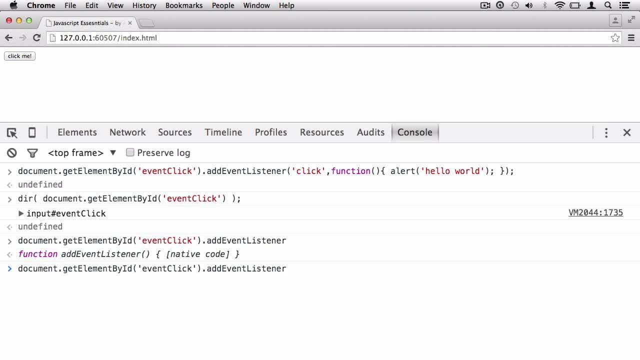 So here's the first one that we added, which was a function that brings up an alert dialogue. Now let's go ahead and add another event listener, And again it's going to be the same: one click And then we're gonna run another function. 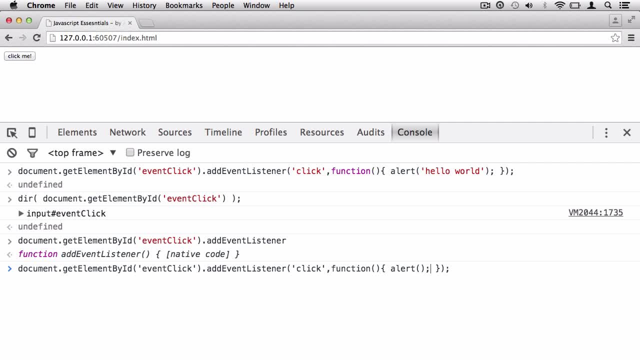 And this time we're gonna create another alert dialogue, which is gonna be another dialogue, like so. So now we're gonna have two alert dialogue boxes when we click on this button. So this function right here does not override or get rid of this function. 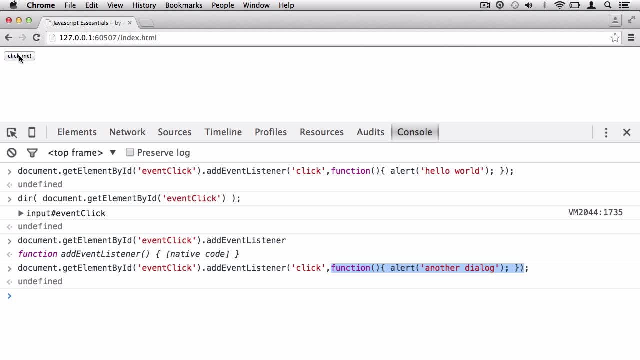 In fact, they are both compiled in memory, So let's take a look at this now click me. We have the first alert dialogue, this one right here, And then another alert dialogue that came from this function down here, So you can have multiple functions. 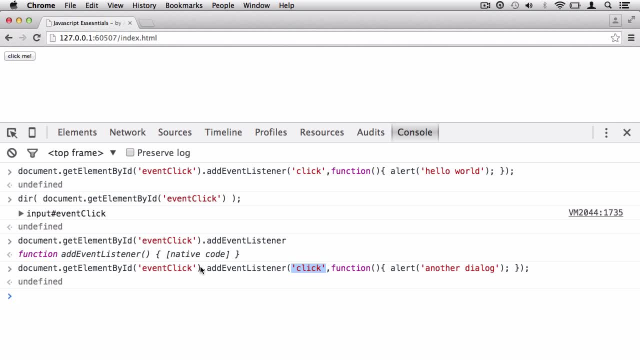 that are attached to a single event on one single element like so. Now I'd also like to show you how to remove events as well, But unfortunately, in this case, I can't actually remove those events. So this is the danger of using the add event listener. 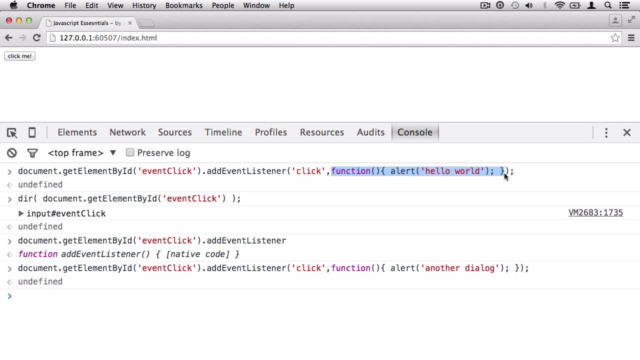 And that is the fact that what I've done is I've added anonymous functions. So, again, these are functions without names, So this function has no name. I can't physically call it back. And the issue with adding anonymous functions or even inline functions with your event listeners: 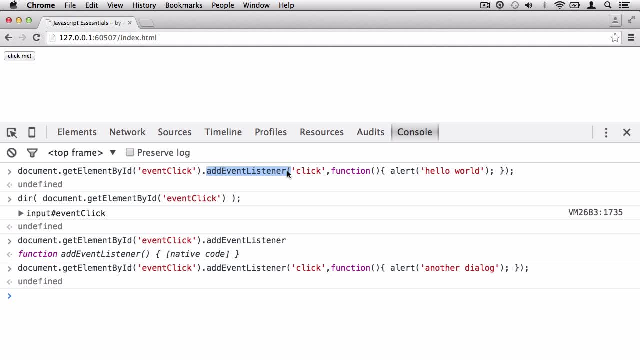 is the fact that you won't be able to remove those functions. You need to be able to reference those functions. so we must create the function outside of the event listener, Because if I was to simply target the element and say, remove event listener, 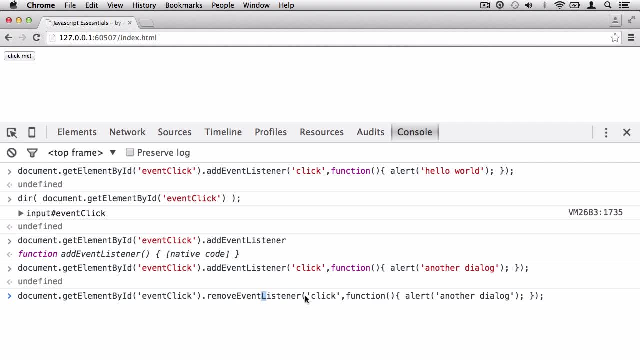 and again: event needs the capital E and listener needs a capital L. And if I was to say, well, just go ahead and remove all of the click functions, for example, no, it's still there, So we can't actually do it. 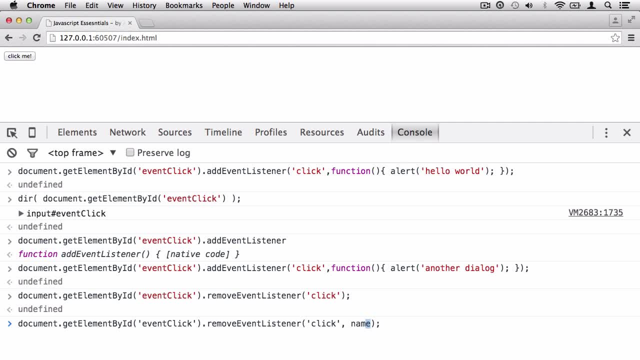 And you do have to define the name of the function that you want to get rid of And, again, this has to be a pointer in memory in JavaScript, So you need to be able to point to it, make a reference to it, which, in this case, 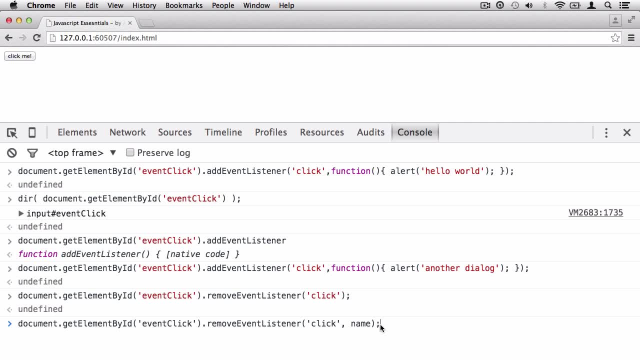 we can't actually do because we have an anonymous function. And likewise, even if I was to give the function a name and you couldn't just say remove event listener and then put a comma in there and then type in name, it still wouldn't work. 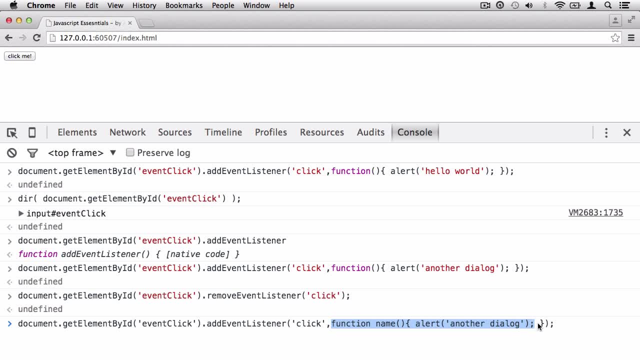 So what you need to do is make sure that this function right here is not actually written in the add event listener. What you need to do is reference it So that function needs to be declared outside of the add event listener method. So let's go ahead and refresh the page and start again. 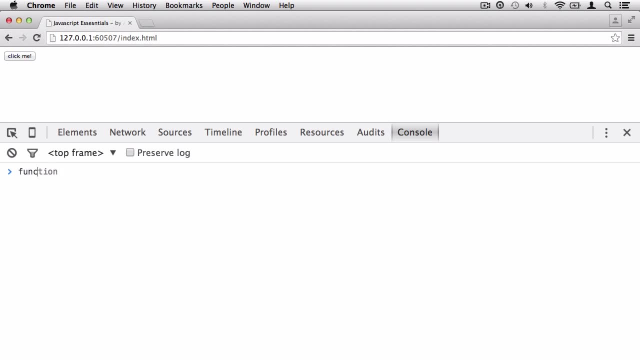 And what I want to do is create a function. Now, this is a globally accessible function, So this function will be stored within a key name in our window: object. Don't forget what happens here if I create a global function, So I'm going to say global function. 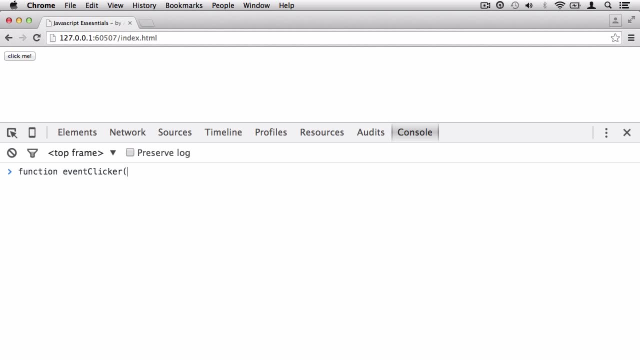 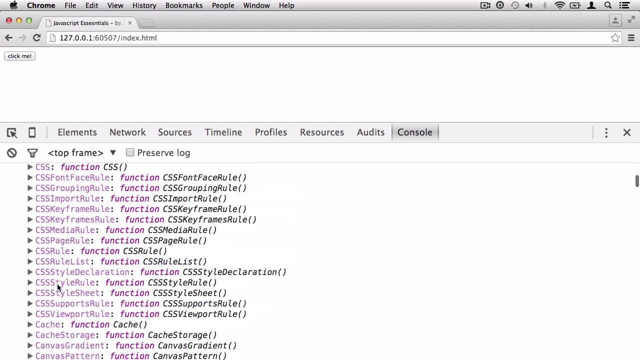 event clicker and then I'm going to open and close the brackets and open and close the parentheses, And the execution context is just going to be one command, which is an alert dialogue box: hello world Now. it will create a key in the window. object: 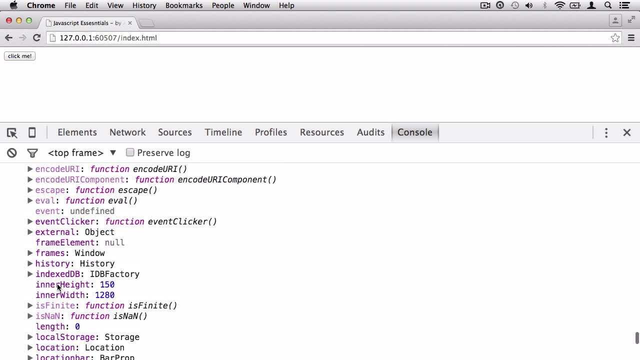 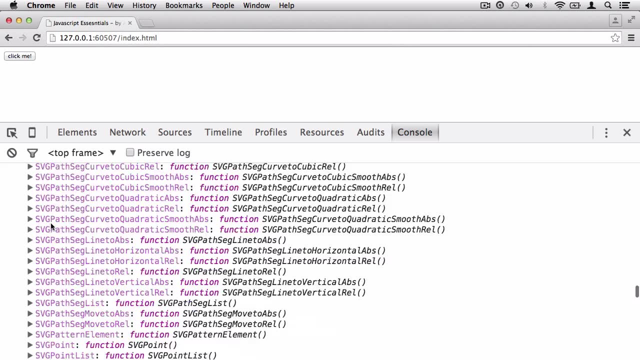 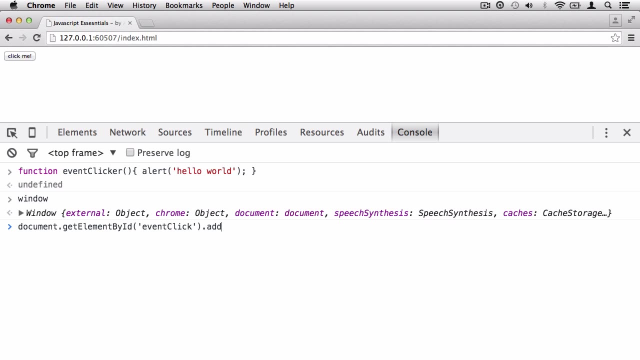 And this key will be called event clicker, And that is a function. There we go, So this is a named function. We can reference this function. So what I can do now is target my DOM element and then I can add an event listener. 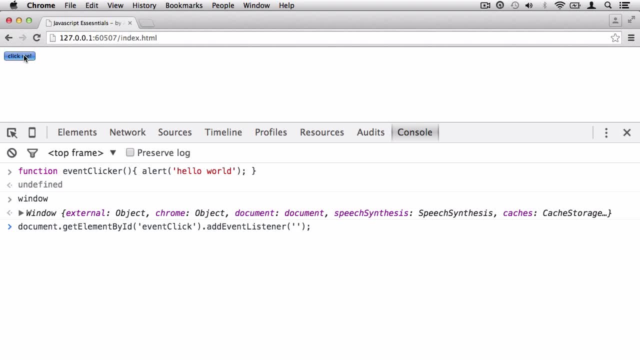 And again, the first parameter is: what event would you like? Well, at the moment, we've got nothing right now, as you can see. So I'm going to add a click event and now I'm not going to write an inline function. 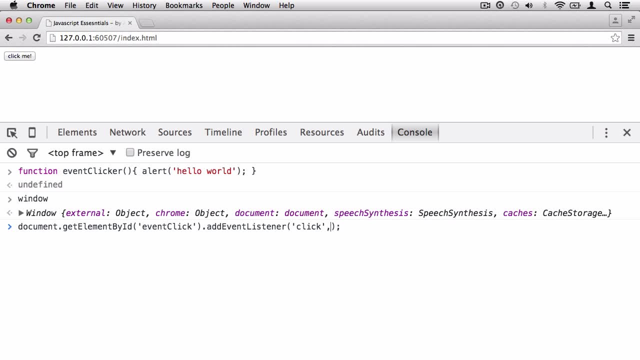 that will be anonymous and be impossible to remove. So what I want to do is reference it. Well, I can reference it by its name: Event clicker. So if I just say event clicker right here, what it's going to do is- JavaScript is pretty smart. 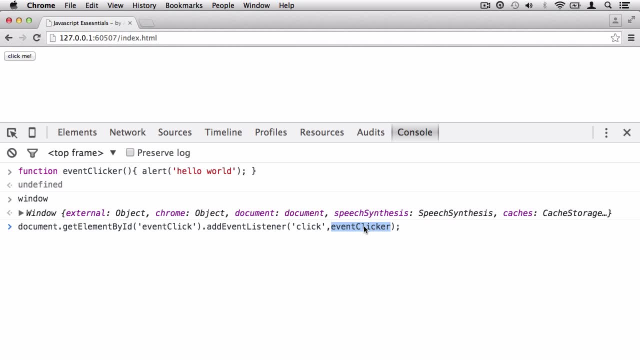 It can say: right. this to me looks like a global, accessible key name, which event clicker is in essence a key name, And it's going to go to the window object and look at the event clicker key and it will find a function.